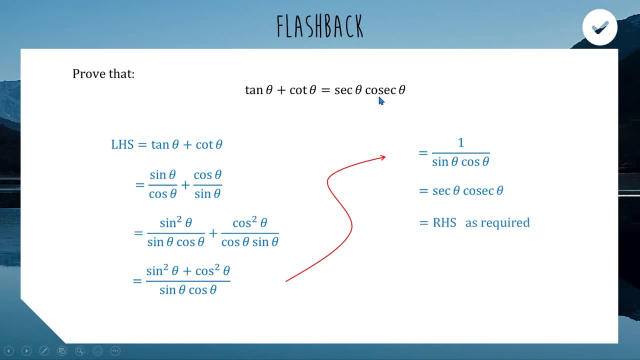 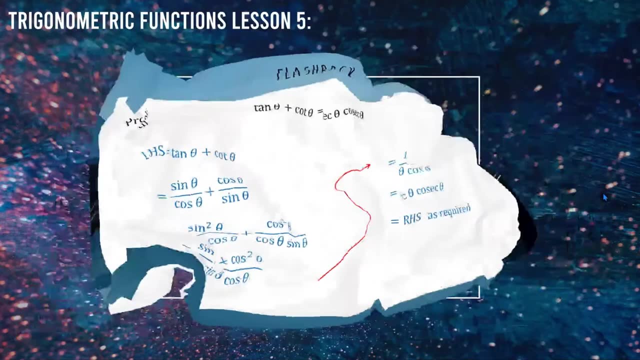 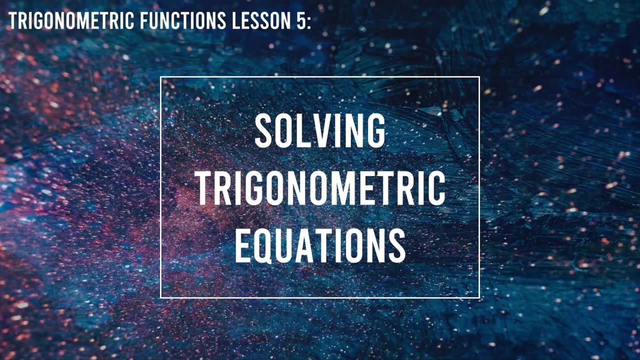 sec theta, cosec theta, which is the right hand side, which was the target. So we write equals, right hand side, as required. Beautiful, All right. today's lesson is on solving trigonometric equations. It's our last lesson in the trig functions topic, which I think you can say. 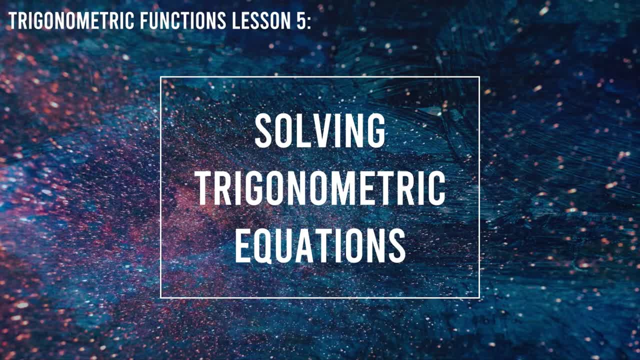 it's been a pretty tough topic. This is also a pretty challenging lesson- Okay, it's one that takes some getting used to. it takes practice, So it's probably going to seem a bit scary at first, but I'll try and go as slow as I can and we'll do some more practice. 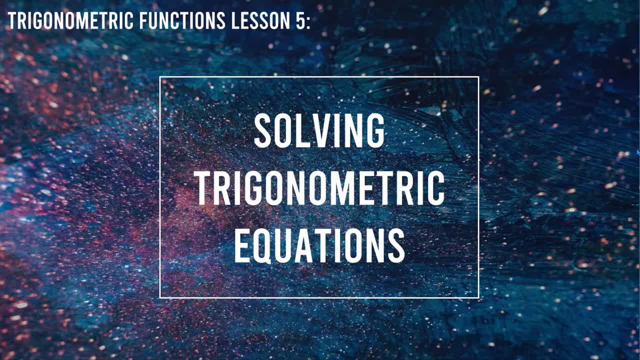 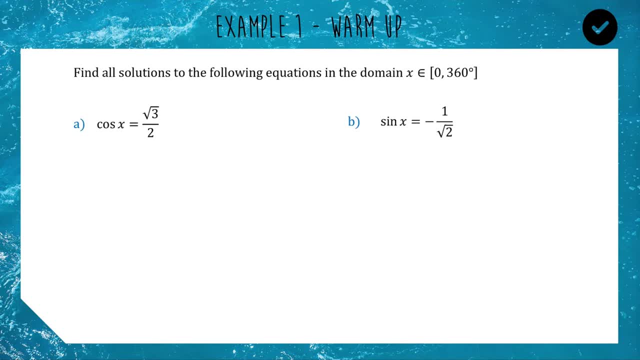 Back in class next week. what a treat. Okay, let's start off with two easier examples just to warm up. So here we are. we have two equations. We are trying to find all solutions in the domain of x as a part of 0 to 360.. So this on the end of the question is some new notation that we haven't. 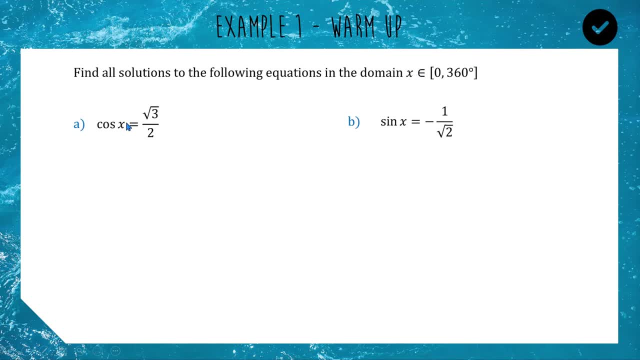 encountered. This is just saying that x, which is what we're solving for. x is the angle, x is a part of the domain from 0 to 360 degrees, So we're going to try and find all solutions in the domain of x as a part of 0 to 360 degrees. 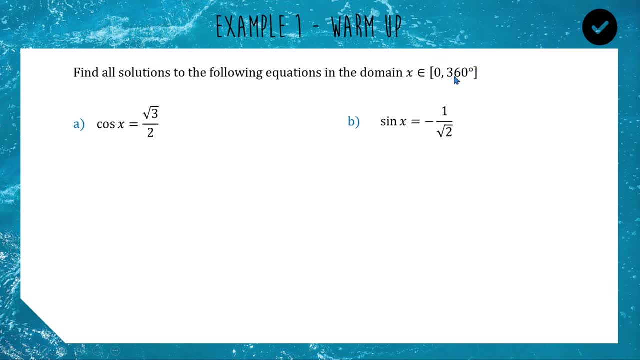 What this really means is just find all the solutions in the first lap of the unit circle. Okay, so this equation right here: cos x equals root 3 on 2,. this is an equation that has an infinite number of solutions, because the graph of cosine wiggles back and forth forever. Okay, we. 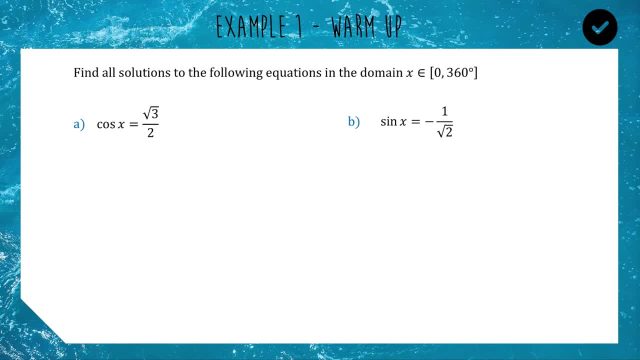 don't want to sit here and find an infinite number of solutions, because we've got more important things to do, So we're just going to find all the solutions from 0 to 360.. Alright, so here's our approach. Usually, the right-hand side of the equation will be: 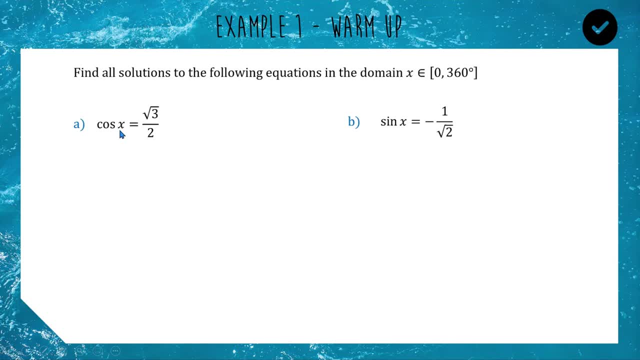 a number that we know some information about- So we have cos of an angle- is equal to root 3 on 2.. As I've said many times in this topic, if you know your exact values from your two magic triangles, these questions become a lot. 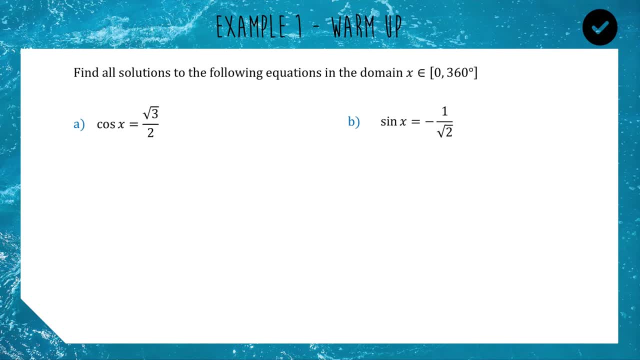 easier, Okay, so the best thing you can do to prepare for this lesson is get your exact values memorized. So if you have them memorized, you know that cos of 30 degrees is equal to root 3 on 2.. Okay, what this tells us is that our solution. 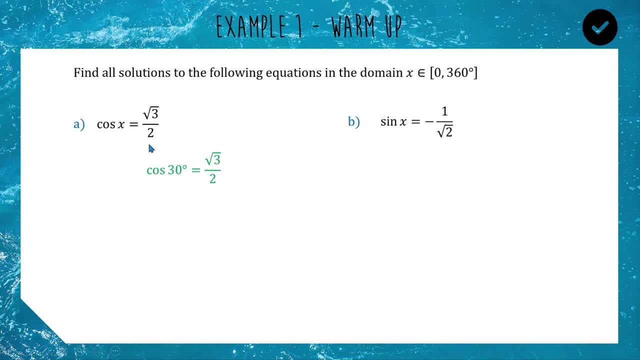 is going to be 30 degrees and it's going to be equal to root 3 on 2.. So if you look at this equation, you can see that our solution is going to be 30 degrees in all the quadrants where cosine is giving us a positive answer. Okay, so cosine is positive. 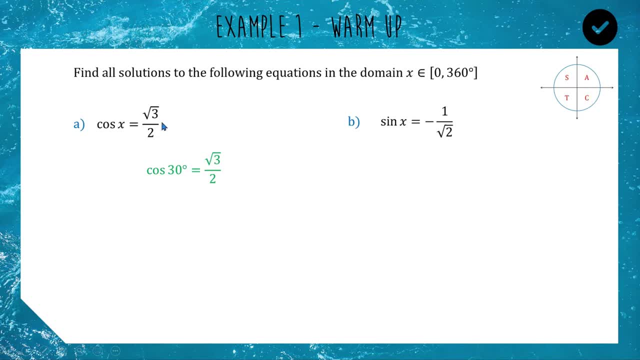 in the first quadrant and the fourth quadrant. So our solutions to this equation are going to be 30 degrees in quadrant one and 30 degrees in quadrant four. Alright, so positive in one and four. So we're going to do 30 degrees in the first quadrant and in the fourth quadrant. 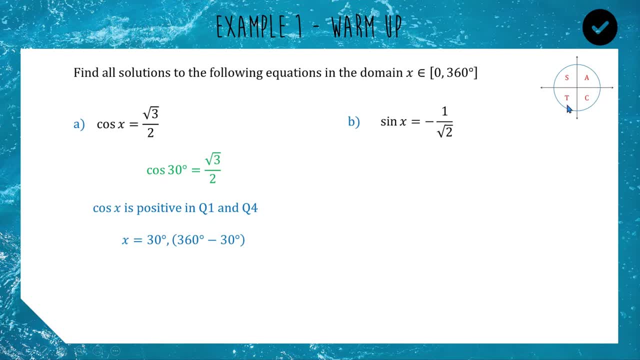 we work back from 360.. Okay so 360 take away 30.. Gets us our second answer of 330.. Okay so if you have your calculator nearby, if you type in cos 30, you'll get the decimal approximation of root 3 on 2.. If you also type in cos 330: 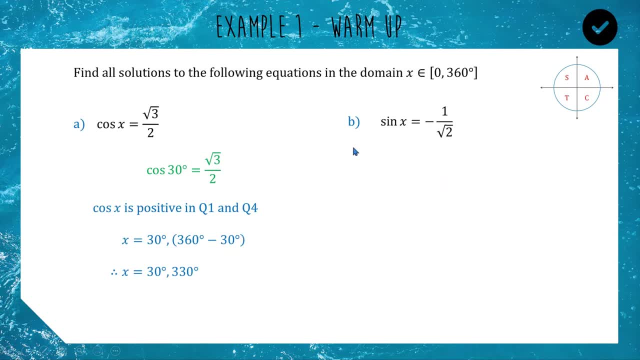 you're going to get the exact same answer because they're the same points on the cosine wave. Okay, I'm guessing that may not have made heaps of sense, but once we do a bunch more examples you'll start to see the pattern and you can follow the steps. Let's have a look at B. We've got. sine. X is equal to minus 1 over root 2.. 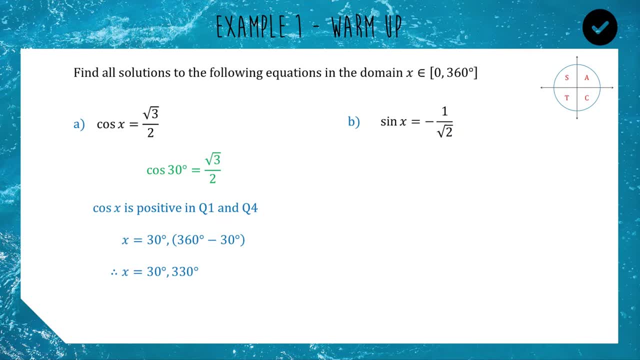 So first thing is we've got to know our exact values and say: well, that's familiar, because I know that sine of 45 is equal to 1 over root 2.. However, the right hand side is negative. What that tells us is we're going to be looking at solutions in the negative. 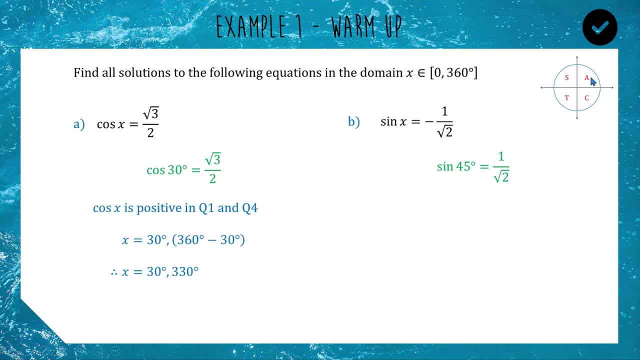 quadrants for sine. Okay, so sine is positive in one and two and it's negative in quadrants three and four. What this tells us is our solutions are going to be 45 degrees in quadrant three and 45 degrees in quadrant four, So we're going to be looking at solutions in 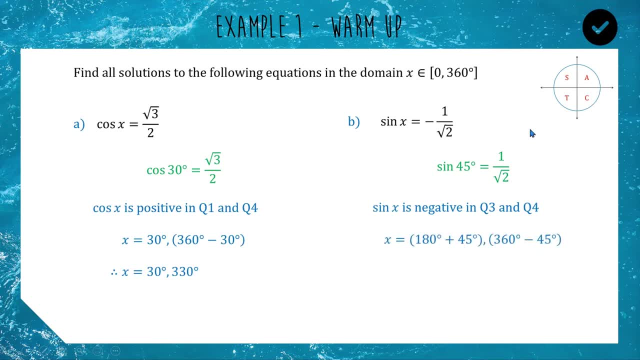 four. Okay, so we're going to be doing 180 plus 45 in quadrant three. In quadrant four, once again, we're going to do 360, take away 45. Gets us our two answers of 225 and 315.. All right, if you put sine of 225 or sine of 315 into your calculator, you'll get the same answer. 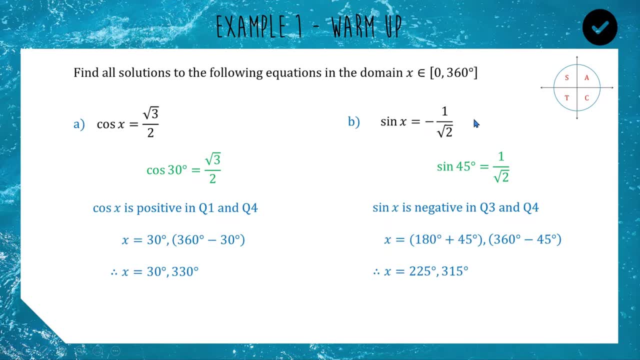 and it'll be a decimal approximation for negative 1 over root 2.. All right, so there's how we figure out our solutions. We figure out which angle we're working with and we figure out which quadrants we're working with. Okay, so once you get the hang of it, it is typically the 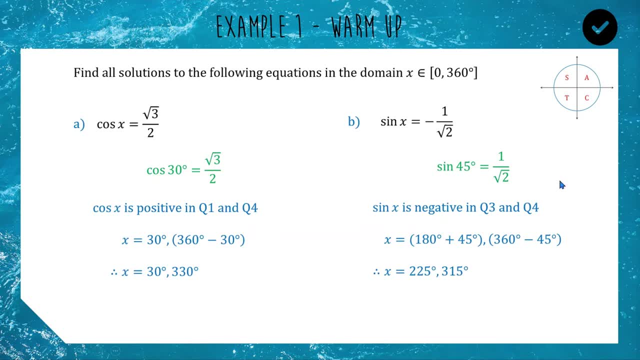 same thing each time. but there are a few tricks to be aware of that. we're going to try and cover all of them in this video. So we're starting off with some level one examples and we're going to move on to some really hard ones later in the lesson. 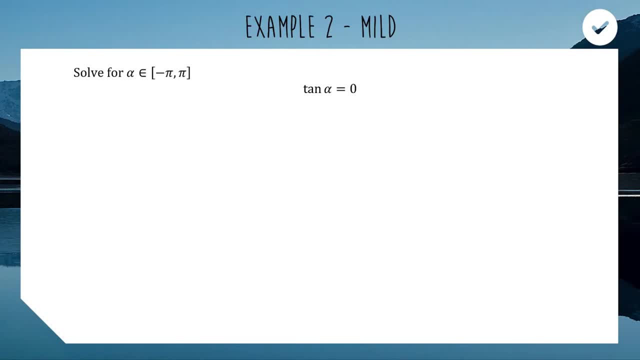 Okay, next up we have a milder example. It looks pretty scary, but there is a nice trick to it. So we're solving for alpha in the domain of negative pi to positive pi, So from negative 1, 80 to positive 1, 80.. The equation we are solving is: tan, alpha is equal to 0.. Okay, so in the last. 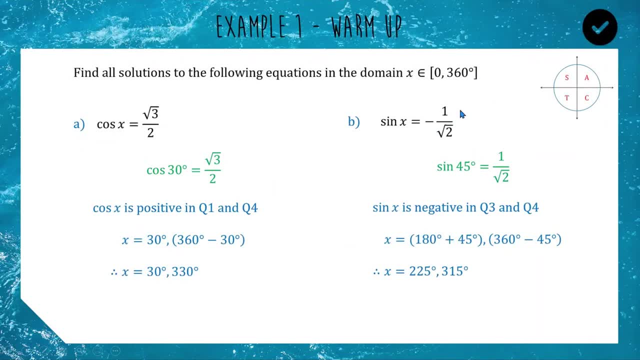 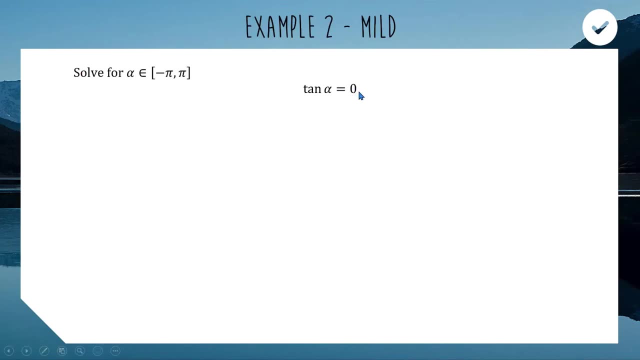 example, we were solving our equal to some fractions that we should recognize from our exact values. When you aren't working with fractions, if you're working with whole numbers like 0 or 1, the knowledge you need to rely on here is your knowledge of sketching. Okay, if you have a good 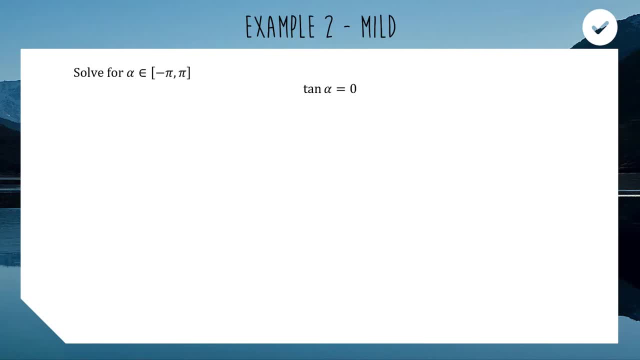 understanding or a good idea in your mind of what sine, cos and tan look like. questions like this can become very simple. Okay, to solve tan alpha equal to 0, we've got to close our eyes and picture our tan lines. Okay, we looked at these in lesson one. Go back if you need a. 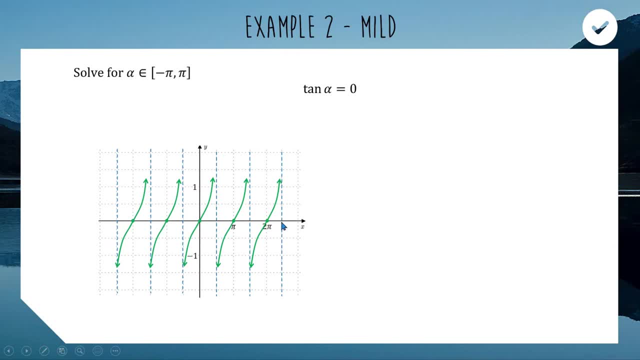 refresher. but this is what tan x looks like over the pretty large domain from minus 2 pi to 2 pi. Okay, so we're solving this, So we're trying to see where is this function equal to 0? from minus pi to pi. So in this region here. Well, where are we 0? Where are we hitting the x-axis? 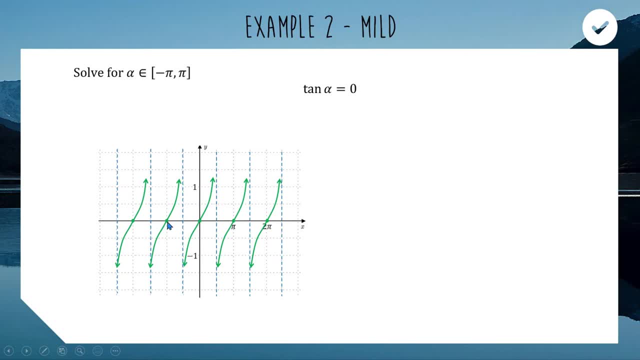 We're hitting at 0.. We're hitting at pi and we're hitting at minus pi. So in this domain we have three solutions and we can see them clearly. if we know what tan x looks like, All right. so if you're equal to 0 or equal to 1, the easiest thing to use is your graphs, typically, especially for sine and 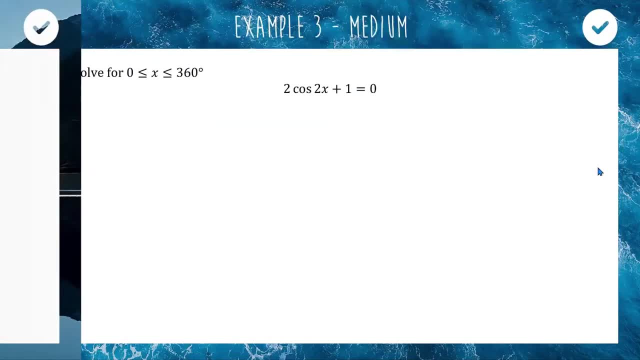 cosine are more common questions. Okay, up next we've got an example I'm calling medium, but it's actually pretty challenging. So medium was a bit optimistic, It's probably more of a tough one. Anyway, we've got 2 multiplied by cos. 2x plus 1 is equal to 0.. Now the aspect of this question. 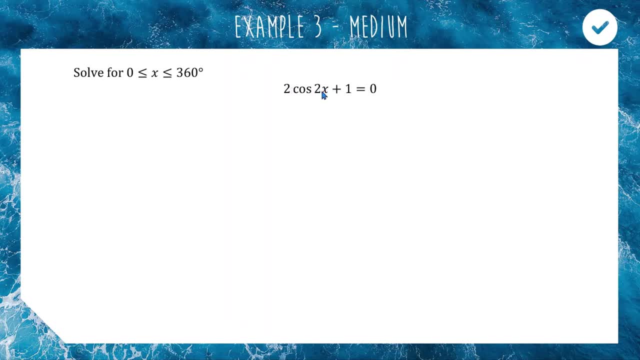 that makes it more challenging is that our angle inside of our cos function is not x, it's 2x. Okay, when you have your angle being multiplied or divided by a constant, it's going to affect your domain. So the first thing to remember here to make this question a bit easier: 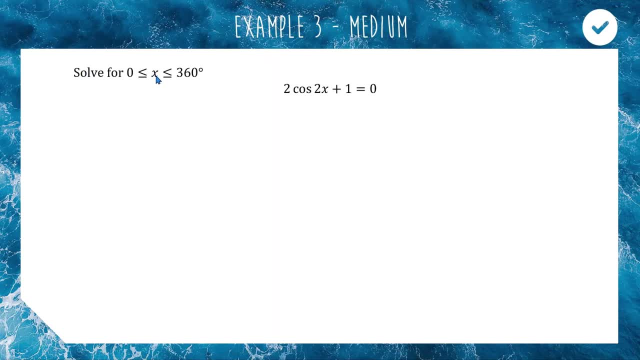 is that, even though the question said we're solving for x in the domain of 0 to 360, if we're analyzing 2x we're going to be solving for x in the domain of 0 to 360. So if x is between 0 and 360, that means 2x is between 0 and 720. So I'm just doubling both. 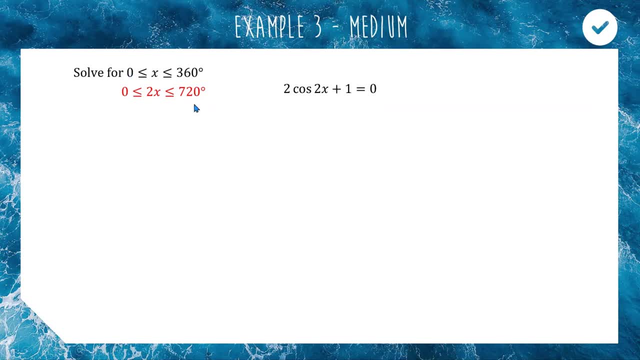 sides, 2 times 0 and 2 times 360.. Okay, remembering this step is going to make sure you get full marks, as opposed to maybe 2 out of 3.. Okay, all right, now let's go ahead and solve this equation like we normally would. We're trying to get everything away from the x, So let's subtract one from both. 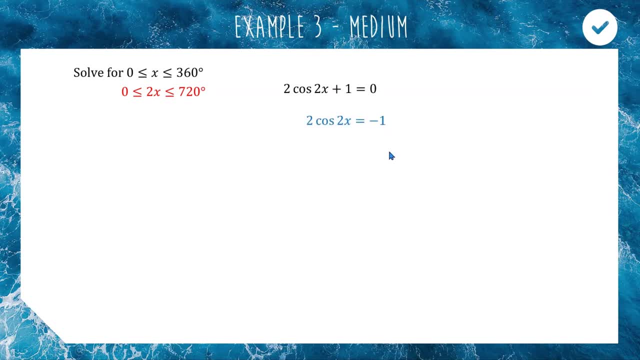 sides to move the minus one across, and now we'll divide both sides by 2.. So we get cos of 2x is equal to minus a half. All right, so we have cos of an angle is equal to minus a half. If we are familiar, 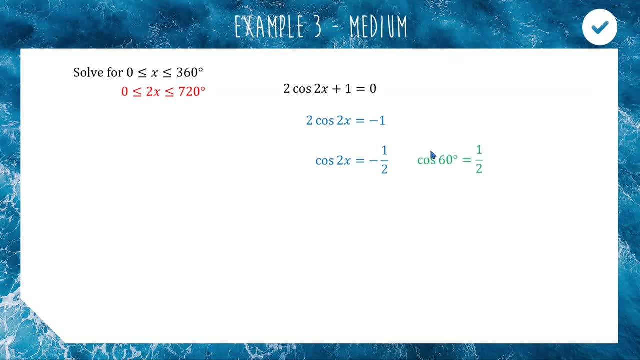 with our exact values. we should know that cos of 60 is equal to a half. What this tells us is that our angle, which this time is 2x, is going to be 60 degrees because we've got a half. So our angle is: 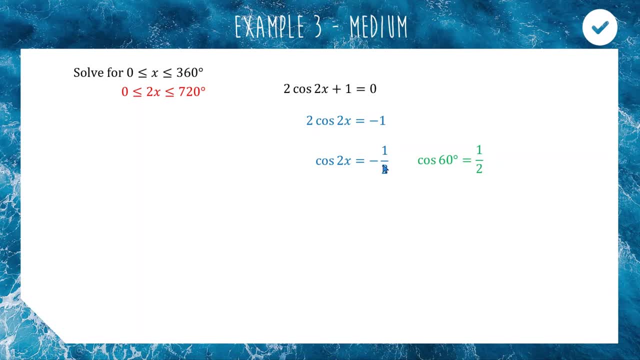 60 degrees and we're going to be in the negative quadrants For cosine. So we'll get our unit circle back. Cosine is positive in 1 and 4. So we're going to be negative in quadrants 2 and 3.. Okay, so our angle 2x is going to be equal to 60, but we're 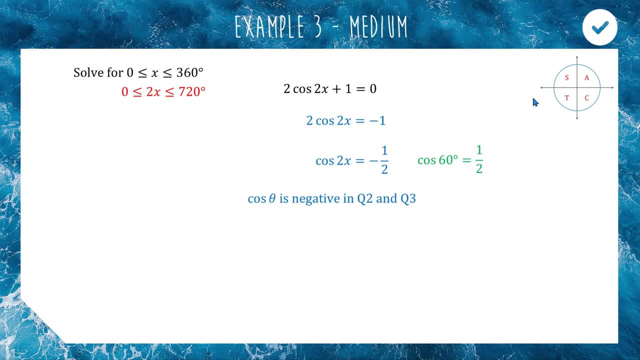 going to be in quadrants 2 and quadrants 3.. Okay, so 2x is going to be 180 minus 60.. That's in quadrant 2, just here, and in quadrant 3 we're 180 plus 60.. I've written some dots here, because there. 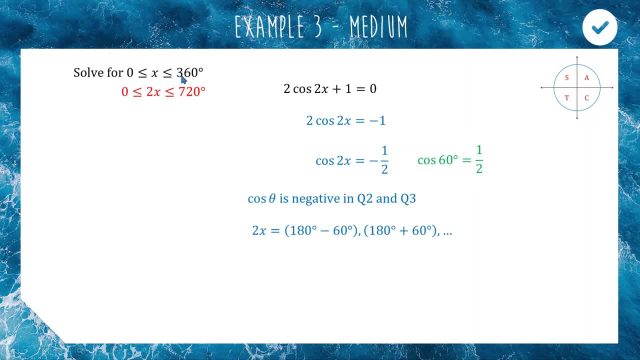 are some dots here and there, So we're going to be in quadrant 3.. So we're going to be in quadrant 3 because, remember, even though x is going between 0 and 360, 2x is going between 0 and 720.. So 2x is 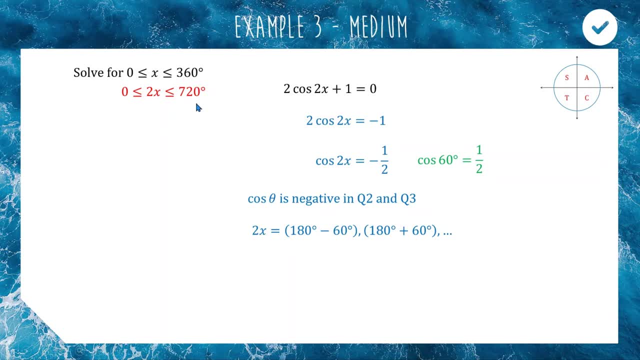 actually doing two laps of the unit circle, But we'll figure that out in a sec. There's a nice trick to getting your extra solutions. All right. so for this one we get 120 and for this one we get 240.. Okay, but like I just mentioned, 2x is doubling our domain and is doing two laps of the unit. 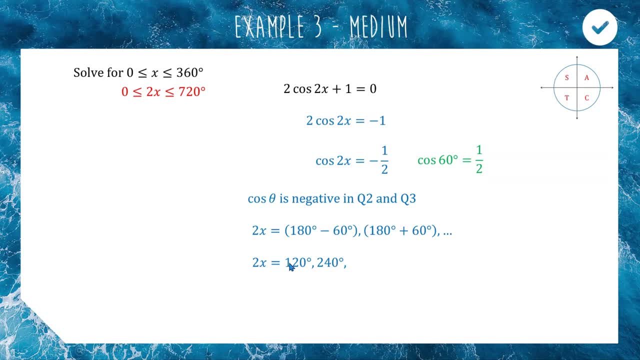 circle. So the way we get the extra solutions is we take our first two, which was in the first lap. we're going to take these two answers and we're going to add 360 to them. So 120 plus 360 is 480 and 240 plus 360 is 600.. Okay, so the 120 and the 240 are in the first lap of the unit circle. 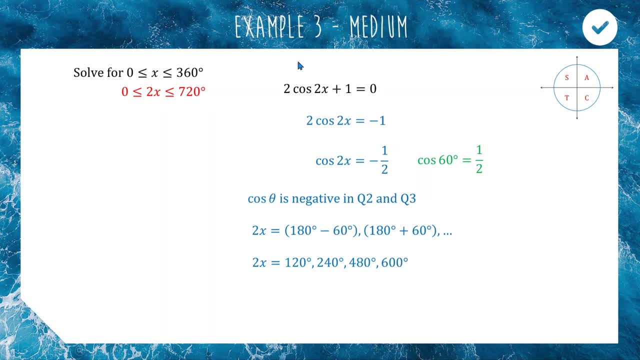 and then 480 and 600 are in the second lap, which gets us up to 720.. Hope that kind of makes sense. We can do more of these next week if we need to. All right, so there's our four solutions for 2x. 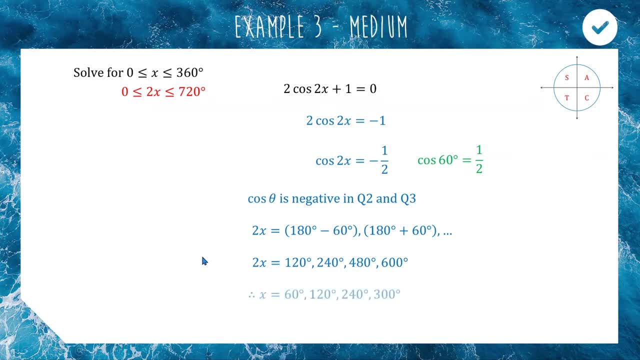 So, to finish off, we're just going to divide everything by 2, so we get our answer for x. So, cutting these all in half, we get our four solutions for x, and they're all between 0 and 360, so they all work out Okay. so if you only get your first, 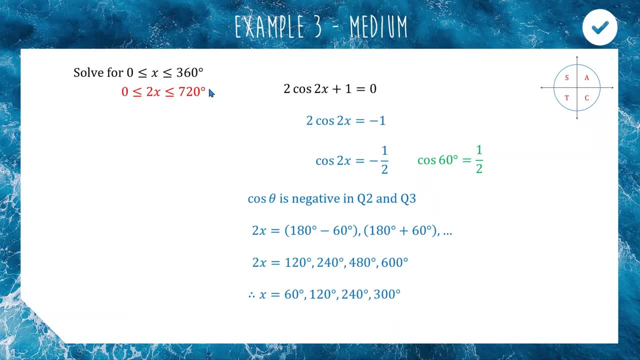 two solutions, because you forget to make this change here, like I said, you're not going to be getting full marks, which is not what we want. Okay, so, lots of steps, like I said, lots of stuff to try and practice and get more confident with. Let's have a go at another one. Okay, up next we. 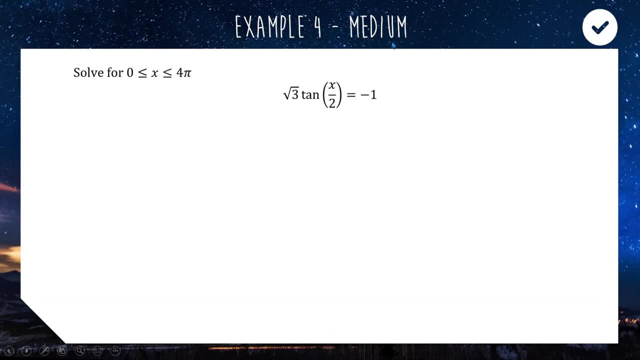 have another example that I very optimistically labeled as medium. In fact it's actually pretty tough, but let's rip into it. So we're solving root 3, tan of x divided by 2 equals 1 in our domain from 0 to 4 pi. All right, so with the last question we had an angle. 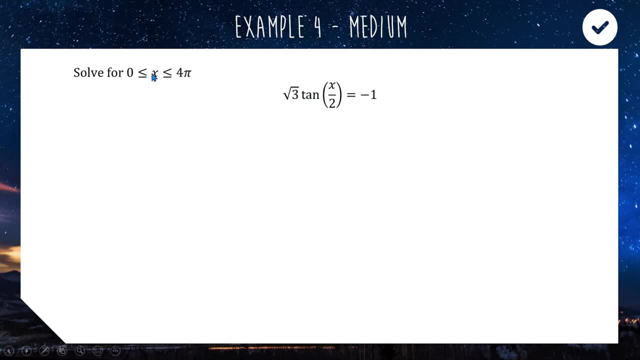 of 2x, and that means we needed to take our domain, which was our x, and we needed to double it. Similar thing needs to happen here. Now our angle is being divided by 2, which means we need to take our domain and we need to cut it in half. All right, so if x is between 0. 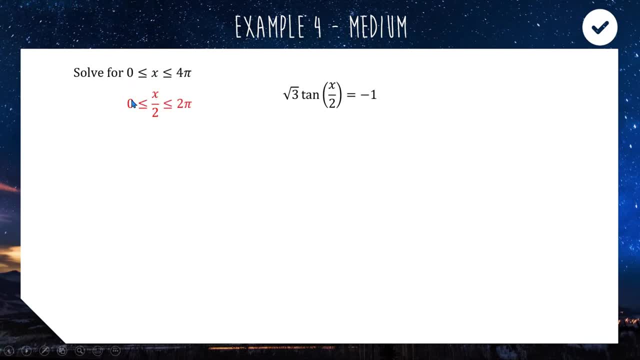 and 4 pi. it means that x divided by 2 is going to be between 0 divided by 2 and 4 pi divided by 2, which is 2 pi. And remember 2 pi is just 360. so this is really just saying one lap of the unit. 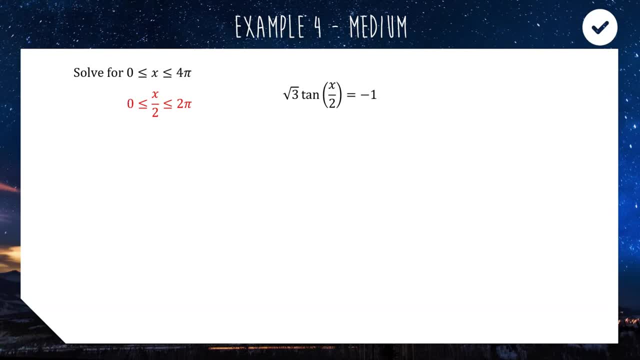 circle. So we've kind of made the question a bit easier on ourselves. Okay, now we can solve the equation. Let's divide both sides by root 3 to get the tan by itself. So we'll get tan of x divided by 2 is equal to negative 1 divided by root 3.. All right, now let's have a go at another one. 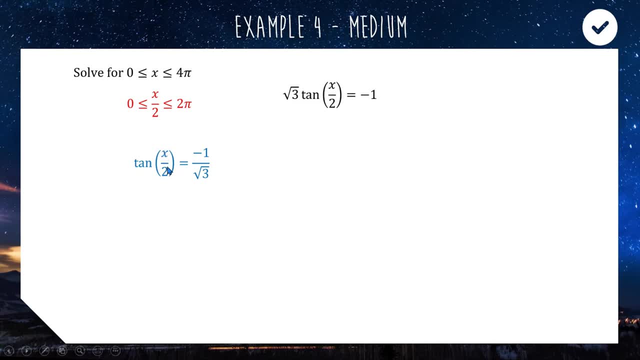 Let's think about exact values. What angle usually goes with tan and gets us an answer of 1 over root 3?? If you're saying 30 degrees, you are spot on. Tan 30 is 1 over root 3.. Okay, we have a negative. 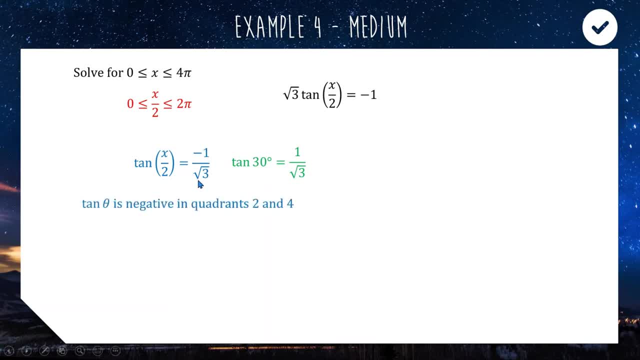 fraction which tells us, for tan theta, we're going to be in quadrants 2 and 4.. Okay so, using our unit circle, again, all stations, 2, central, All right, so 30 degrees and we're going to do 30 degrees in quadrants 2 and 4.. So in quadrant 2 we subtract from 180.. 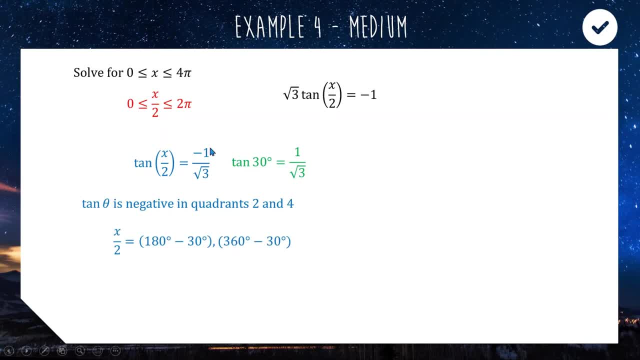 And in quadrant 4 we subtract from 360.. All right, so we're getting our answers for our angle, which is x over 2.. Okay, so 180 minus 30 turns into 150 and we get 330 just here. Okay, excellent. Now we're going to take our two answers, because these are for x over 2.. We need 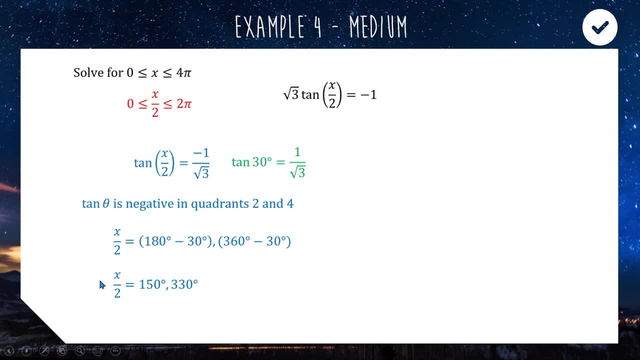 to multiply everything by 2 to get just x. Okay, so we're trying to go from x over 2 to x. So we're going to double our two answers. So we're going to double our two answers. So we're going to double. 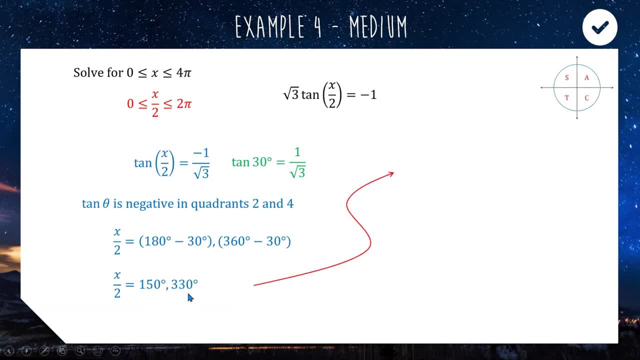 our two answers, Which gets us 300 degrees and 660 degrees. Okay, so 150 times by 2 and 330 times by 2.. Now, extra trick, like I said, because our domain was given to us in radians, the way we are expected to. 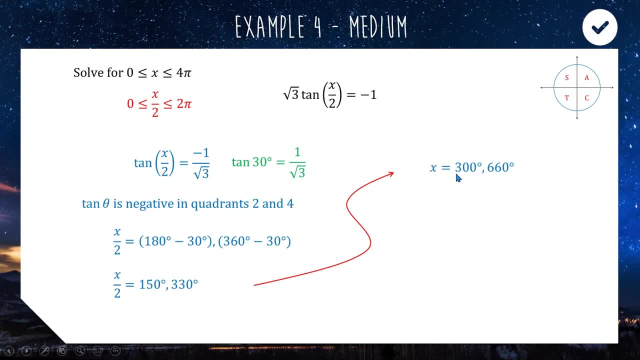 leave? our answer is in radians. Okay, so if you leave your answer in degrees, when your x was given to you in radians, you're risking not getting full marks. So to finish this question off, we need to write 360 in radians. So we whack a pi with them and divide them by 180.. So now they're in radians. Now we simplify our 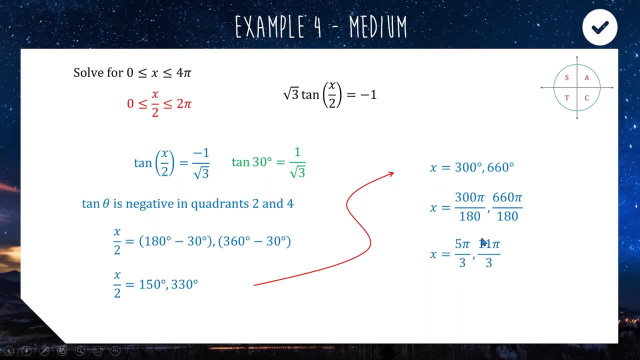 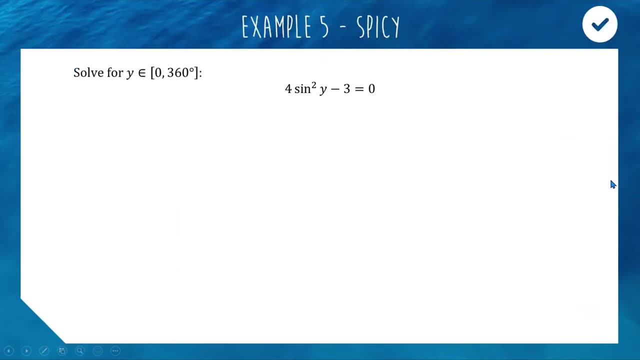 fractions, and we get five-thirds of pi and we get eleven-thirds of pi- Cool. so there's our steps. So remember, the important step is changing your domain so you get the right amount of solutions. Cool, All right up. next we're on to the spicy level of equation We have solving for y in the 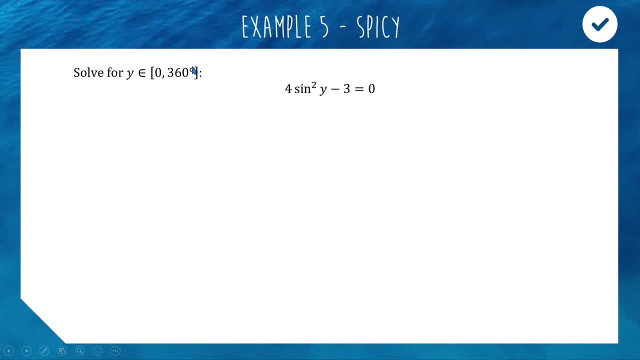 domain of 0 to 360 degrees. So we're going to do that. So we're going to do that, So we're going to give it a look at our own numbers. So we're going to say we have a 1 over y in degrees. So one lap of 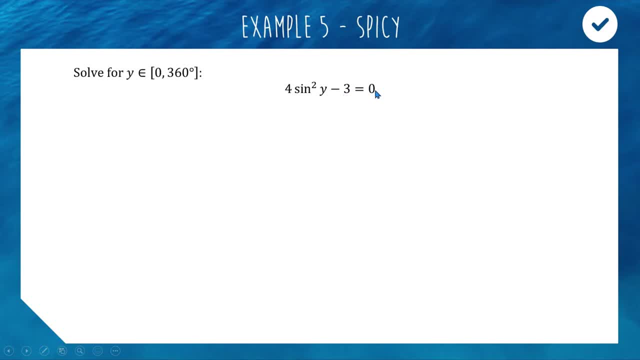 the unit circle and we're working in degrees. We've got 4 sine squared minus 3 is equal to 0.. So now, instead of working with signs, we're working with sine squares, which makes things a little bit more challenging. Okay, let's solve the equation, Let's try and get the sign by itself, So we're. 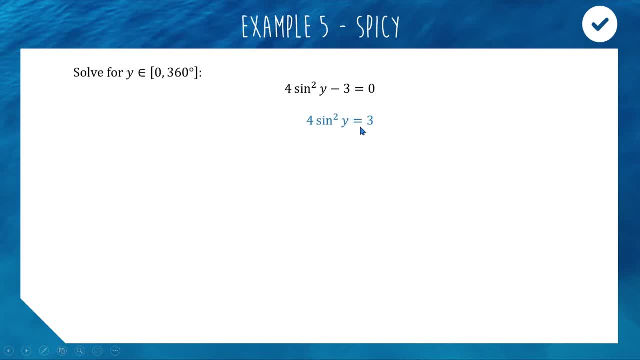 going to add the 3 across to the right-hand side. Now we can divide both sides by 4 to get rid of the 4 multiplying. Okay, now, keep in mind, We are trying to get sine y, yeah. So how are we going to get rid of sine squared? 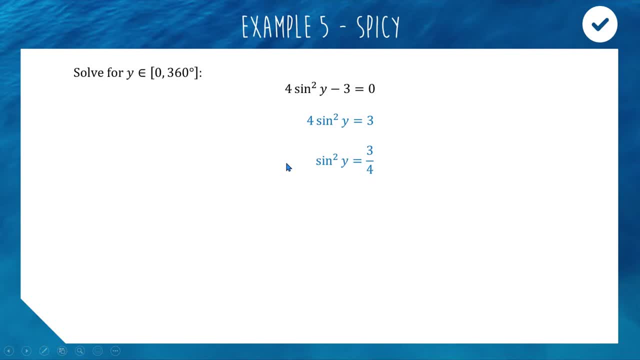 Well, usually the way we get rid of a squared in mathematics is we do a square root, And whenever we do that in an equation, what do we need to remember to do? Hopefully, you are thinking plus minus, So we're going to take the square root of both sides. 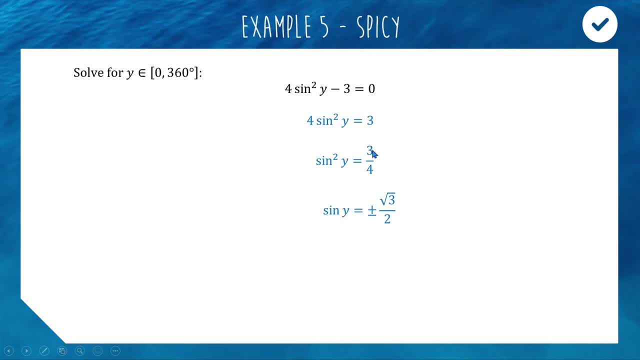 Okay, so the square root of sine squared is sine. Square root of 3 is square root of 3.. Square root of 4 is 2.. And don't forget your plus minus Very, very important. Okay, now we need to have some exact values, knowledge. 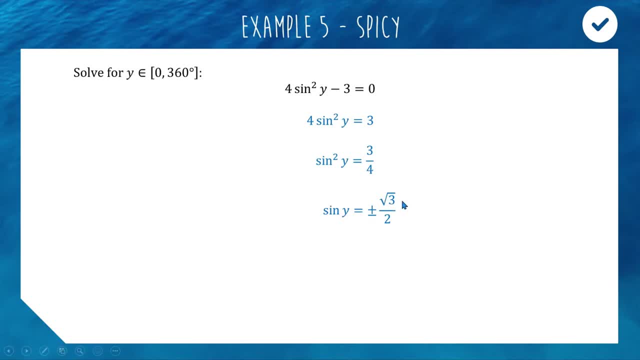 So what angle is typically going with sine and giving us an answer of root 3 on 2?? If you're thinking 60, that is correct. Alright, so 60 degrees. The interesting thing, though, is that the right hand side is both positive and negative. 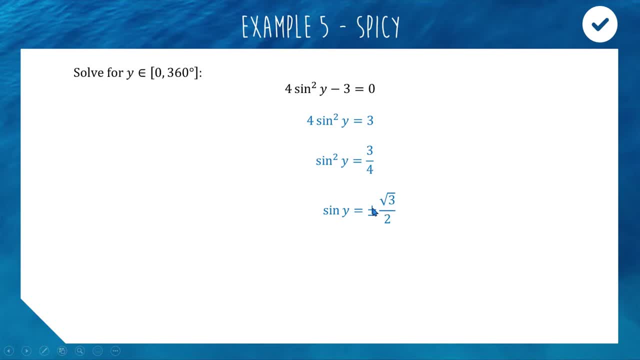 So, in terms of our four quadrants ASTC, because we're positive and negative, we're going to be in all four quadrants, Alright. so sine 60 is root 3 on 2. And because we've got a plus minus. 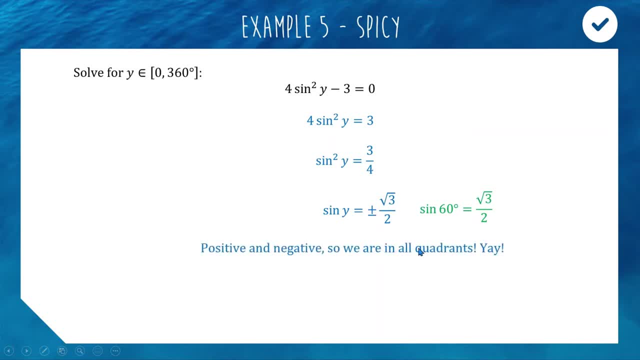 we're going to be in all four quadrants, So everyone gets a turn, Alright. so we have 60 in quadrant 1,, 60 in quadrant 2,, 60 in quadrant 3, and 60 in quadrant 4.. 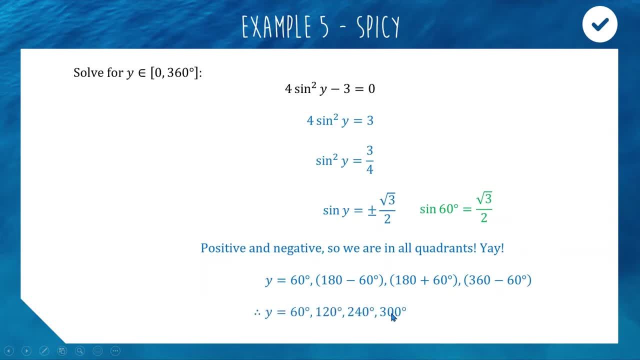 Gets us a final answer of 60,, 120,, 240, and 300.. Okay cool. So the trick for this question was: if you've got a sine squared, you can get a sine by doing a square root. Just don't forget your plus minus. 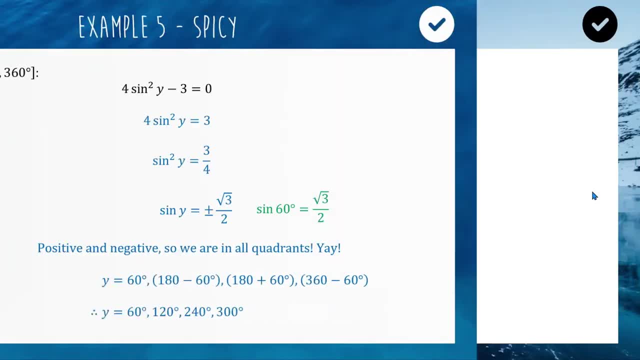 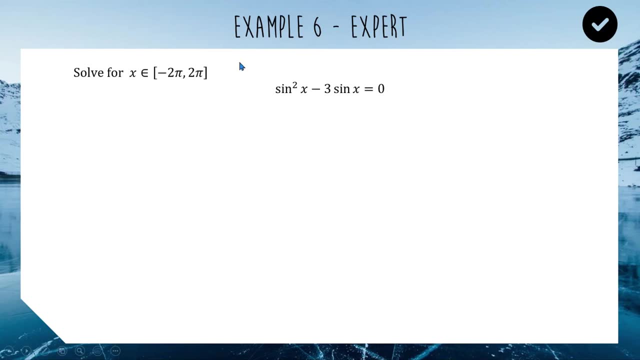 so you get all of your solutions. Okay, on to our second, last example. now an expert level equation we have. We're solving x in the domain of minus 2 pi to 2 pi, So from negative 360 up to 360. 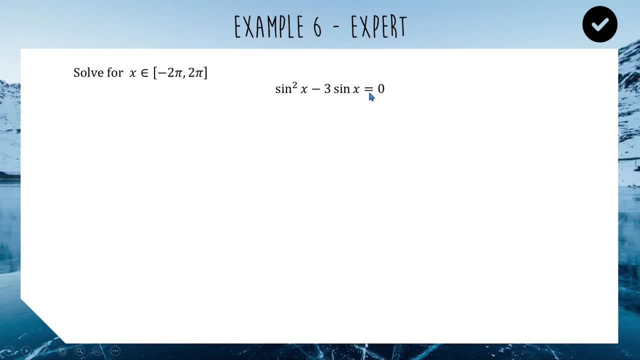 Our equation is: sine squared: x minus 3 sine x is equal to 0.. Now, last equation: we had a sine squared which we could figure out by doing a square root. This one, we have a sine squared and we have a sine. 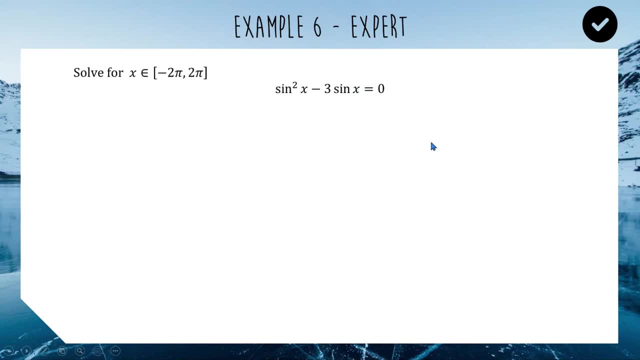 So we have something squared and we have something here. The way to handle this equation is we've got to kind of take a step back and sort of see this as a quadratic equation. Okay, think of this as like x squared, take away, 3x is equal to 0.. 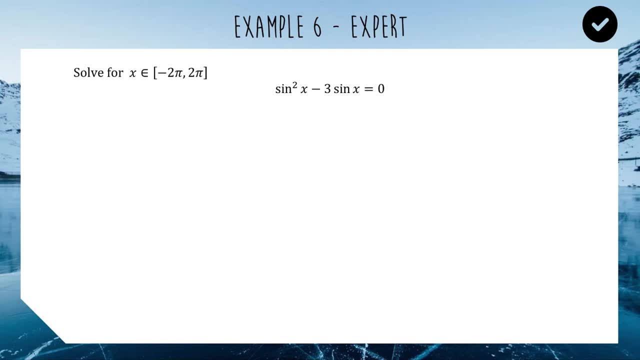 Okay. the way we would solve an equation like that very simply is by factorizing. That's what we're going to do here. We have: the front term is a sine squared, and we have 3 times sine. So we have a common factor of sine x. 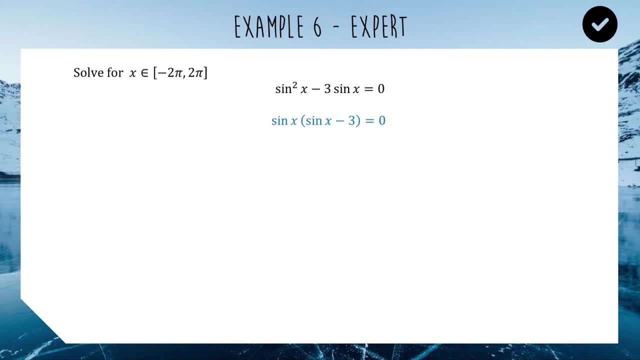 I'm going to factor that out, the front of the expression. So we've got sine x outside of sine x. take away 3 equal to 0. Now we have two things multiplying giving us an answer of 0. We know from quadratic equations. 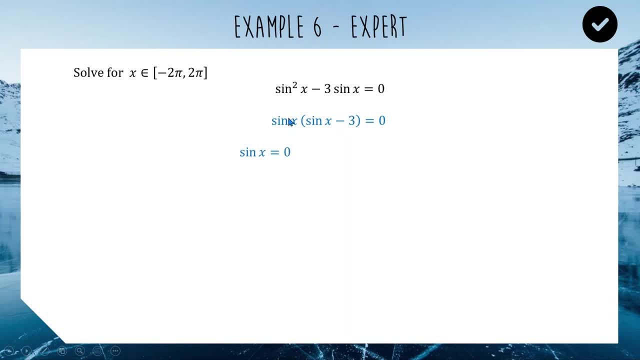 this means that either piece could be 0.. So either the sine x is giving us the 0 or the sine x minus 3 is the 0.. All right, so sine x minus 3 is equal to 0.. If we add the 3 across: 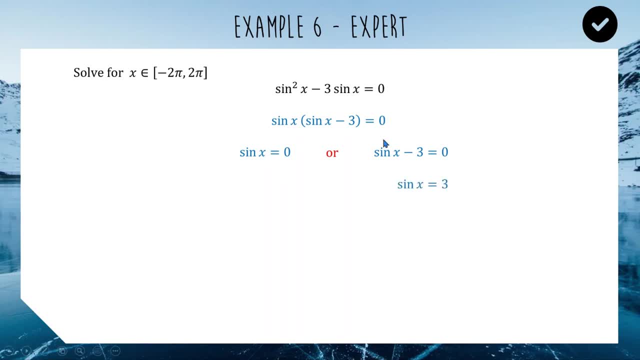 we get that sine x is equal to 3.. Okay, both of these, because they aren't our magic fractions. we need to rely on, once again, our knowledge of what a sine curve looks like. So if you can do a quick, 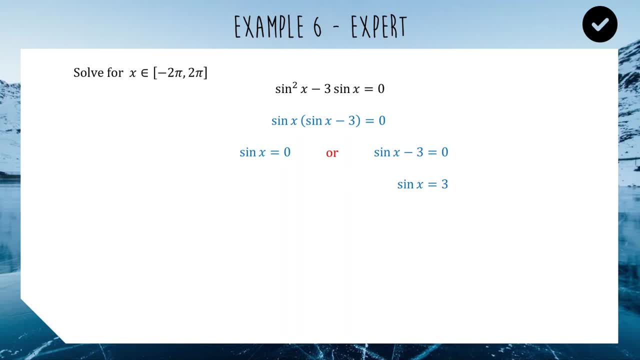 quick scribble, or maybe you can picture it in your head if you've got a really good memory. this is what our curve of sine x looks like. All right Now, when we're seeing where it's equal to something, we're looking at the height of the function. 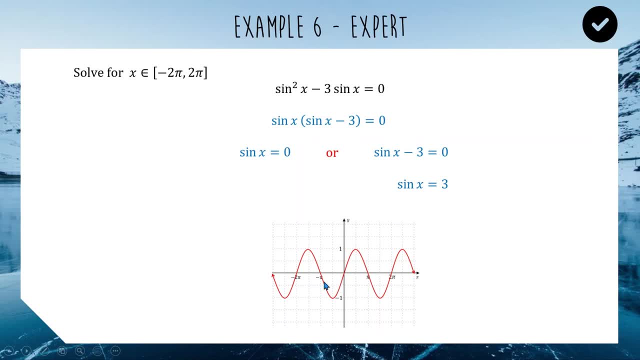 which is the y value. So, first of all, where is this curve reaching a height of 3?? Well, we can see pretty clearly that it's never going to do that, because the height of the curve never goes above the maximum value. So, first of all, where is this curve reaching a height of 3?? Well, we can see pretty clearly that it's never going to do that, because the height of the curve never goes above the maximum value. 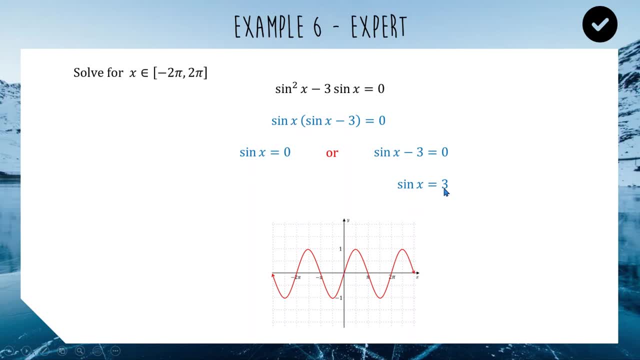 So, first of all, we can see pretty clearly that it's never going to do that, because the height of the curve never goes above the maximum value of 1.. So if you're trying to solve sine x equal to 3,, this has no solutions. 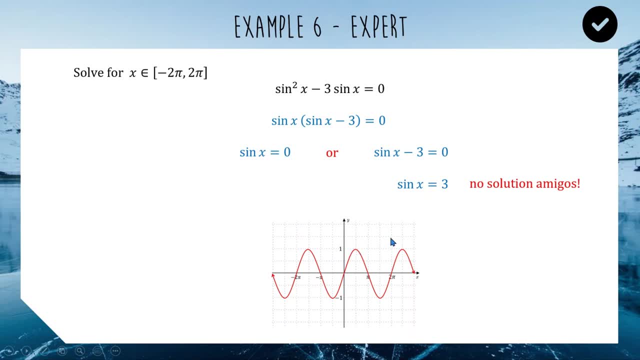 Okay. The curve never reaches a value of 3, unless it's being multiplied by 3, which is not Okay. So anything outside of 1 or minus 1 for sine x will have no solutions Over on the left-hand side. 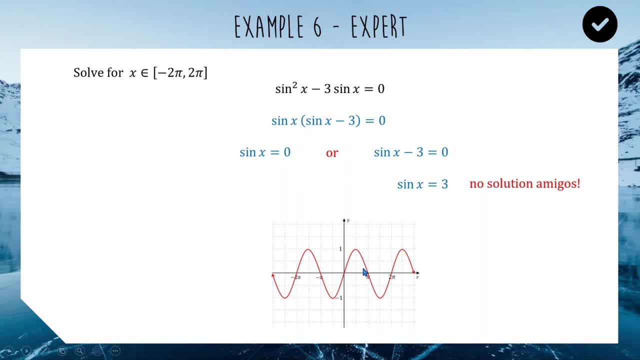 sine x equal to 0, that's our x intercepts and we can see we have quite a few of those, From minus pi to 2 pi. our solutions are going to be minus 2 pi, minus pi 0,. 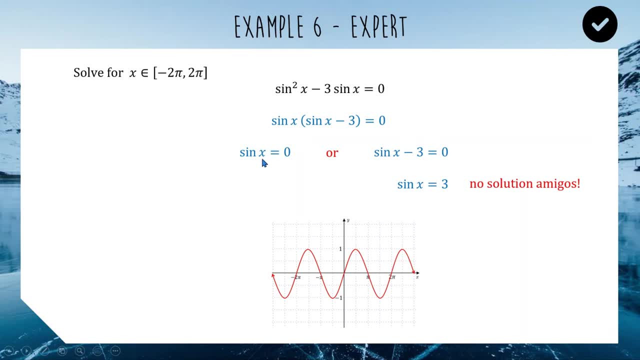 0,, 0, pi and 2 pi. Okay, So solving equal to 0 is finding your x axis intercepts, which is right here. Of course, we should write them in radians, because our domain is in radians, Okay, 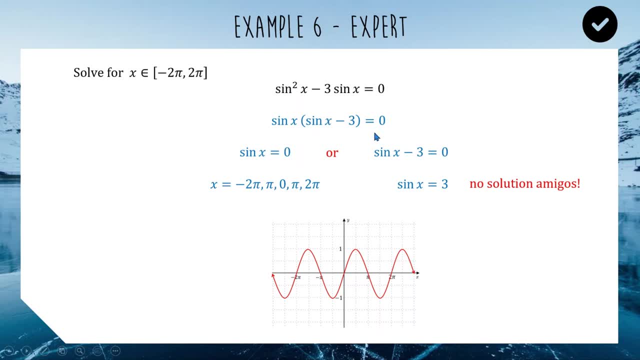 cool. So yeah, you can factorize using trigonometry, You can solve quadratic equations using trigonometry. And don't forget, knowing what your sketches look like can make seemingly hard questions. Very, very simple. Okay, Onto our final example. 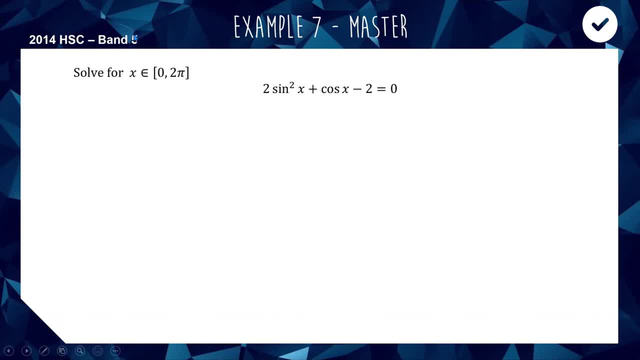 Now this is from a HSC question. It's a band five, So it's pretty challenging. So this is a master level question. We're solving from 0 to 2 pi. Our equation is: 2 sine squared x plus cos x take away 2 is equal to 0.. 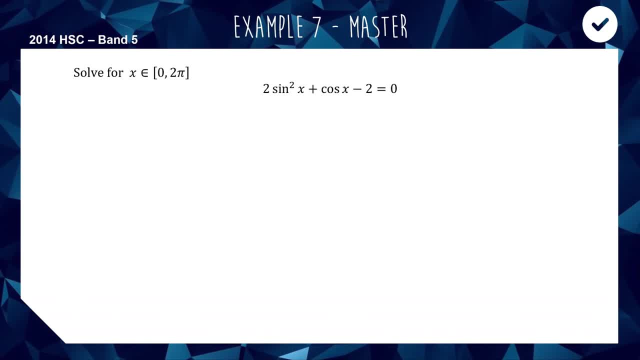 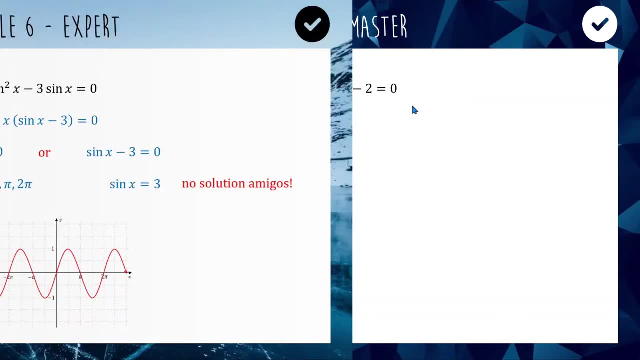 All right, let's have a think why this one is significantly more challenging than the last one. Well, first reason is because we have a constant as well, So we have a more complicated equation. With the last one, we had a sine squared. 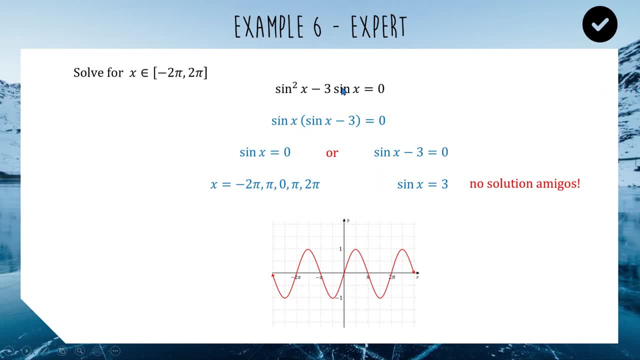 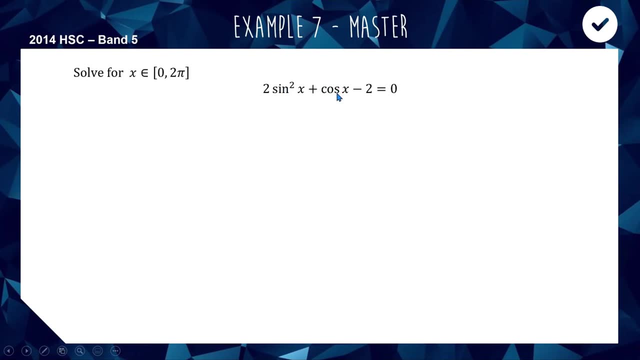 but we also had a sine. So it already kind of looked like a quadratic equation that we could do some cool algebra with this one. We've got a sine squared but we've got a cos x right here. So if we had sine squared and sine, 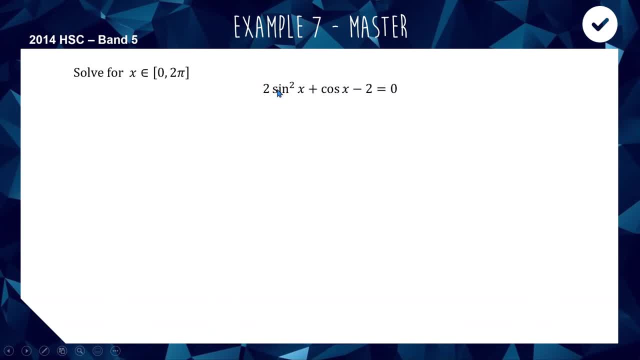 we could turn this into a quadratic equation and do some cool stuff, But because these pieces don't match, we can't do that. So we've got to be really clever and we've got to turn one of these into a sine or a cos. 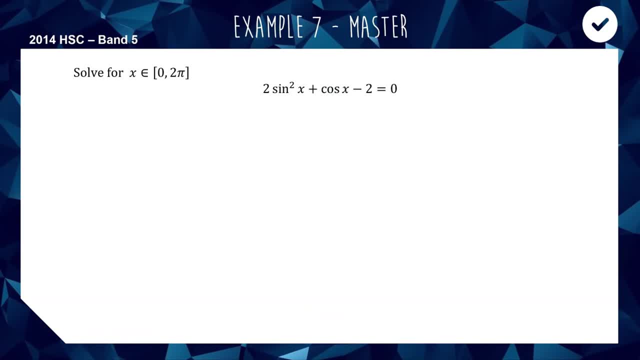 The way we're going to do, that is, we're going to rely on our old faithful Pythagorean identity, which is: sine squared plus cos squared is equal to one. Okay, we're going to rearrange this like we've done before and say: 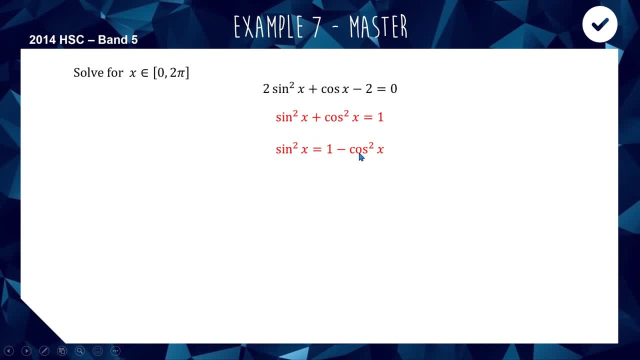 well, this means that sine squared is equal to one takeaway cos squared. Why is that important? Well, because now we can change the sine squared in our equation to a one minus cos squared, And now our equation will be in terms of cos as opposed to one of each. 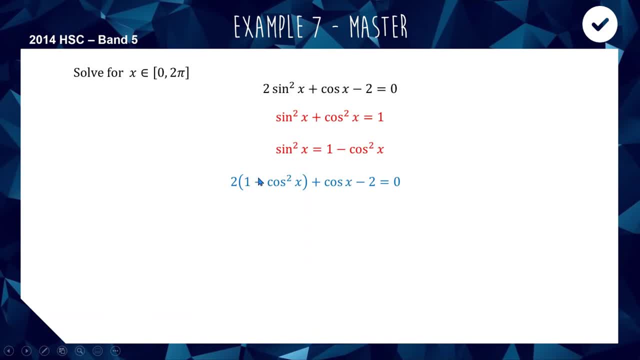 Okay. so we're going to take our equation, we're going to change the sine squared to a one minus cos squared and we're going to expand this out and simplify as best we can. Okay, so we get two minus two cos squared, plus cos x, minus two equal to zero. 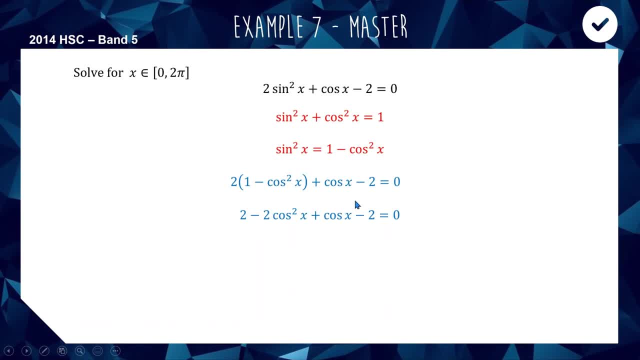 which is already pretty convenient, because we've got a two at the front and we've got a minus two on the ends and those two are going to cancel out and leave us with minus two. cos squared x plus cos x is equal to zero. Okay. 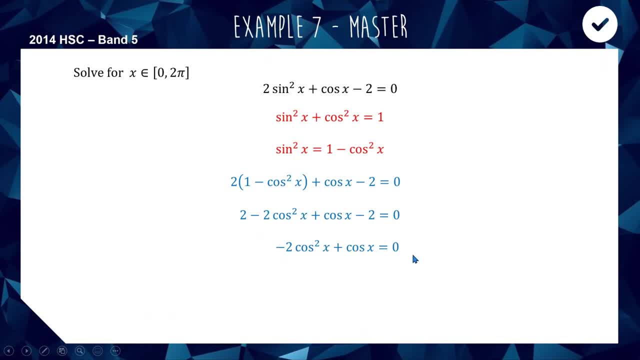 now we're at the point where we're looking, similar to the last question, where we can do some factorizing and solving Okay. so the key to this question is recognizing that these two don't match, but you can make them match by doing some clever algebra. 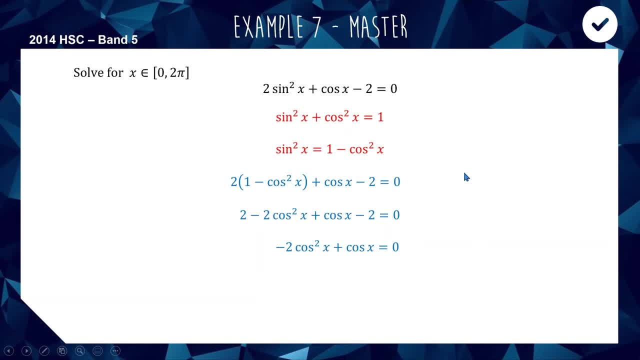 which is why this is a band five question, because not many people would know to do that. Okay now, a quadratic equation is always easier when you're leading terms. So your squared term is positive. So what I'm going to do now is I'm going to multiply everything by negative one. 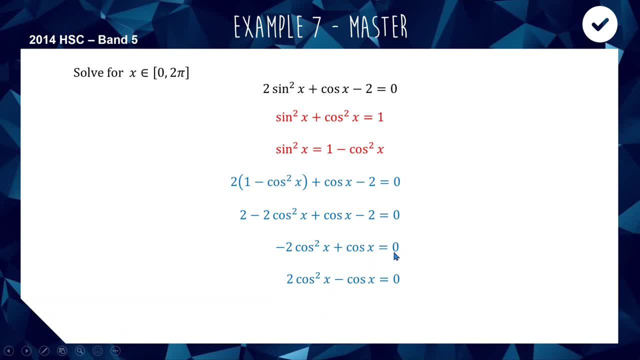 makes our front term positive, makes our second term negative, and zero is still zero. Okay, now, like last time, we're going to factorize this expression, because we have a common factor of cos x. So factoring cos x out the front. 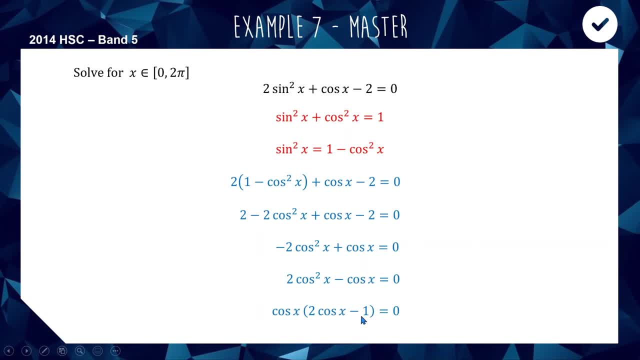 we get two cos x for our first term minus one for our second term equal to zero. Now from this line, we can get two equations. We'll get: the cos x is equal to zero, or two cos x minus one is equal to zero. 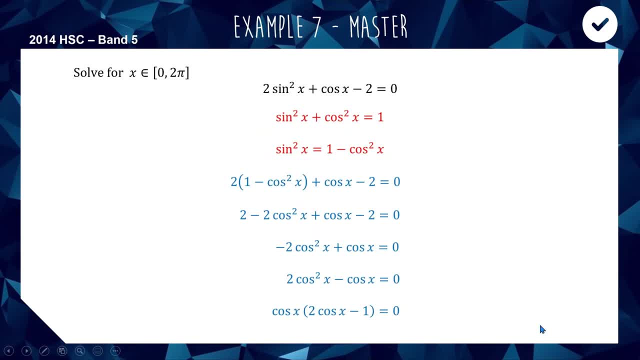 Okay, so there are two equations that we just got from our bracket to terms at the end. So now cos x equals equal to zero. We're going to solve that using our knowledge of the cosine curve, and this right hand one we're going to solve as an equation. 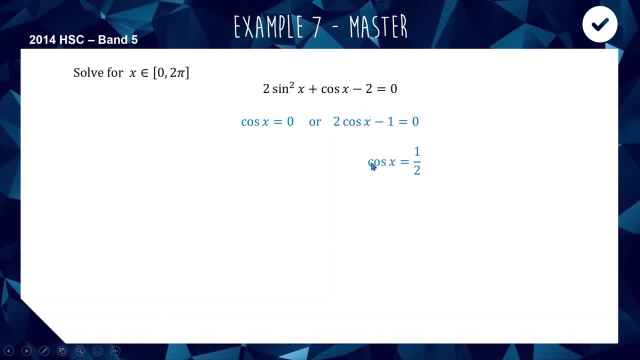 So we're going to add the one across and then divide by two. So we get cos x equal to a half, equal to positive a half, which is important, All right. so if the left hand one cos x equal to zero, if we know what the cosine curve looks like, 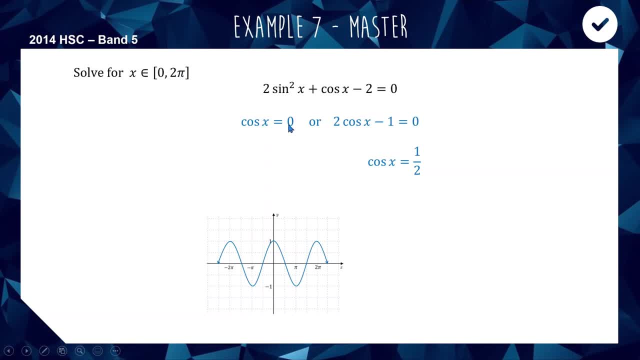 we can see that from zero to two, pi cos x is equal to zero, at pi on two and three, pi on two, So 90 degrees and 270 degrees. All right, so there's our solutions for the cosine curve, The left hand. one: for cos x equals zero, for cos equal to a half. 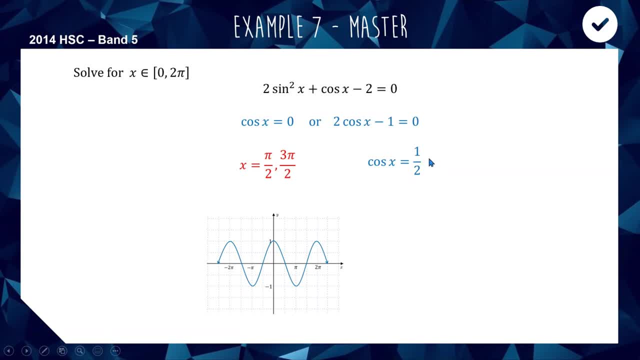 We know that cos 60 is equal to a half. So we're going to be doing 60 degrees in the positive quadrants for cosine, which will be quadrants one and quadrants four. Okay, so 60 degrees in quadrant one gets us a half and 60 degrees in quadrant four also gets us positive a half. 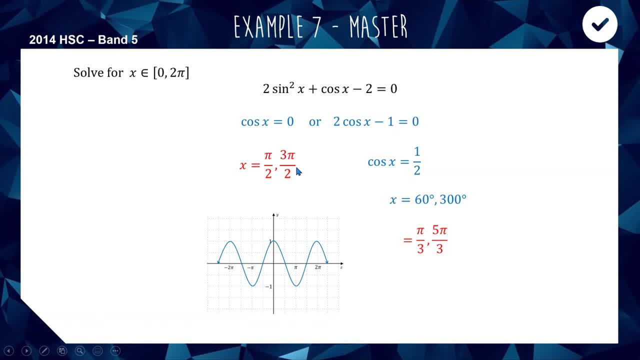 We'll turn these two answers into radians And there we have our four solutions. So x is equal to- I didn't finish it off How lazy. x is equal to pi on three, pi on two, three pi on two and five pi on three. 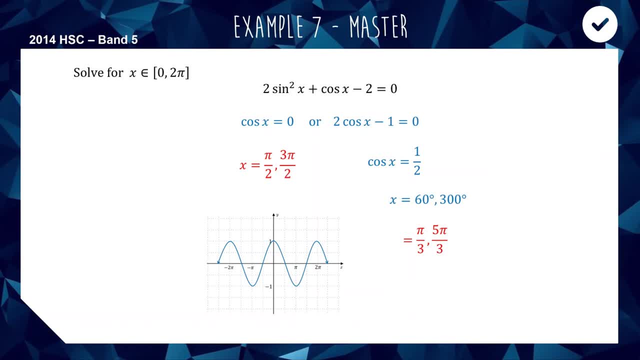 Okay, so lots and lots of steps. That was a three mark question, which is why there's quite a lot of work to it. We may not be at this level yet, but maybe when we're doing some revision later in the topic. 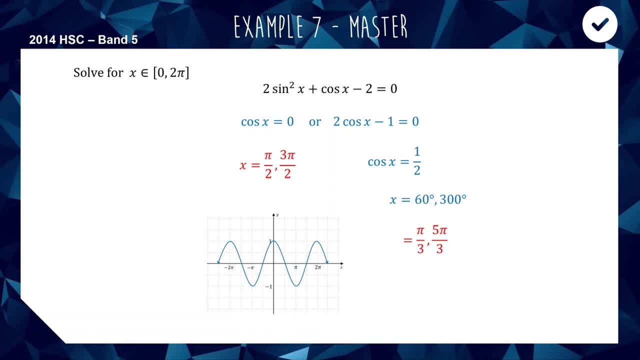 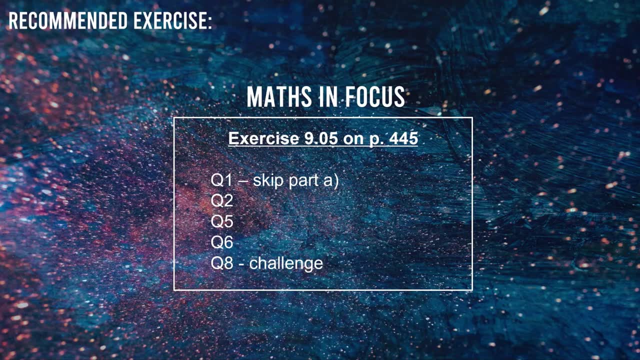 we can try some more tough questions like this one. Okay, thanks so much for watching that. I hope some of it makes sense. We'll do some more practice later on. as I said, because it's very challenging, Here's some practice for you guys to have a go at now. 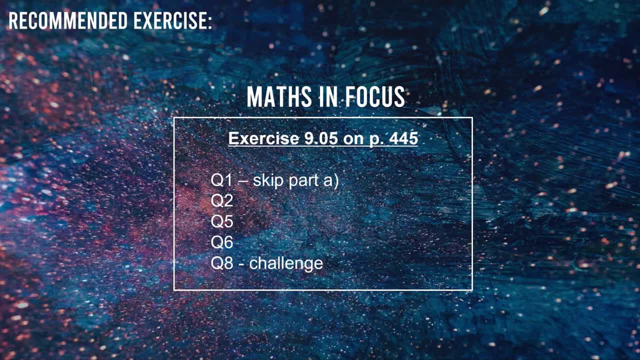 and we can build upon this next week when we're back in class. Thanks for watching this lesson. I'll see you guys later on.